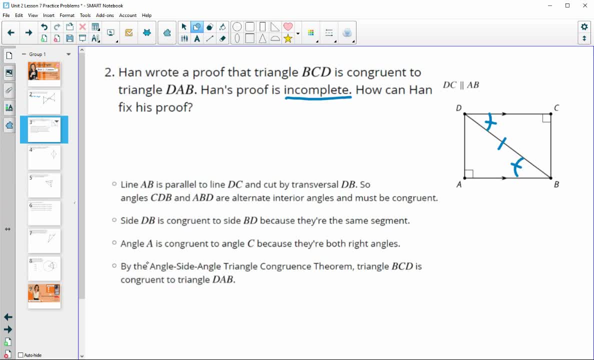 So this is where he is missing something, because right now, as he has it on his picture, he's not showing That the triangles are congruent by angle side angle, because he doesn't have the side between the two angles. 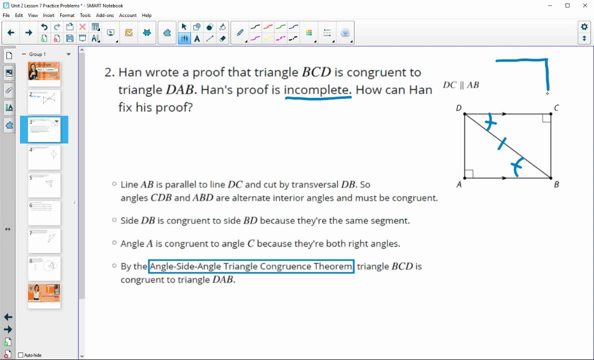 So what we actually do know is that within one triangle he knows two of the angles. So he knows this one and he knows this one, And that's the same in this other triangle has a right angle and then this same measurement. So what he needs to do here is add in a step. 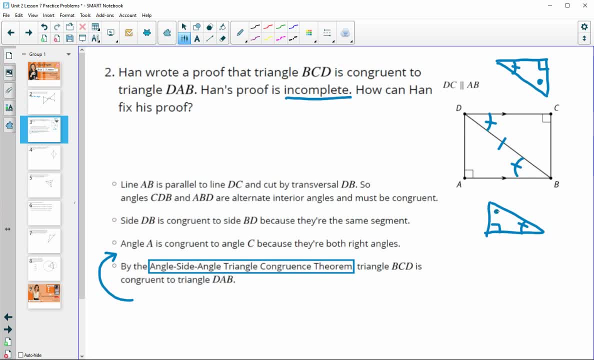 To say how he actually knows that this angle is congruent to this angle. Because once he does that, once he proves that this angle is congruent to this angle, then he has angle side angle, because he'll have it here and then he'll have this side in between. 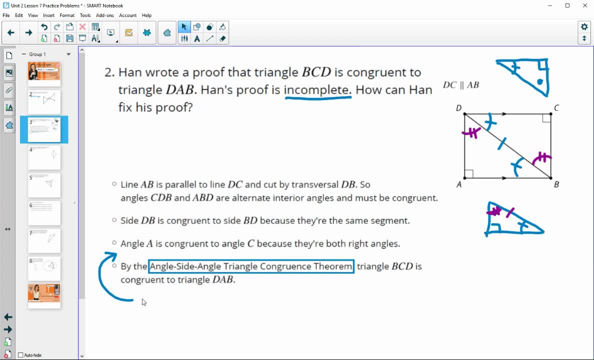 So we just need to add in this step here that by the triangle- some theorem, It's all triangles, It's all triangles, It's all triangles. Add to 180 degrees. If you know two of the angles are the same, then the third one has to be the same too. 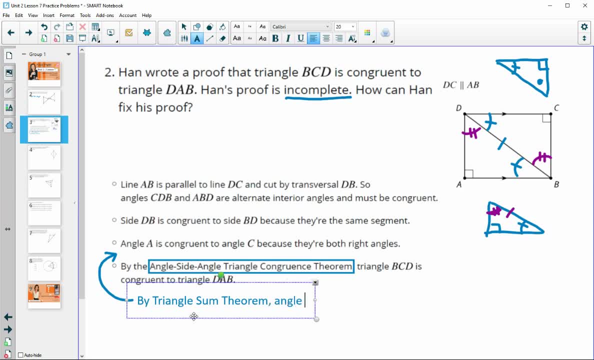 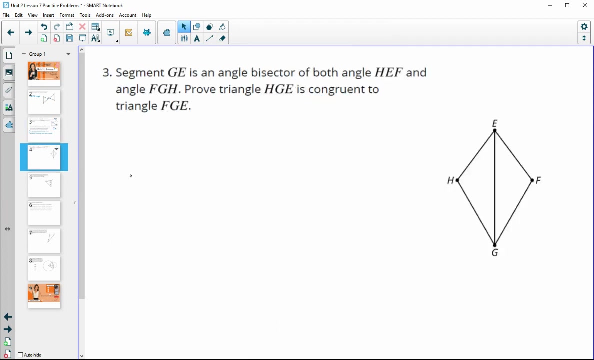 So by triangle, some theorem, angle CBD is congruent to angle ABB. Just add that in before that final step, Then he would know by angle side angle that the triangles are congruent. Number three, segment GE, is the angle bisector of both angle HEF and FGH. 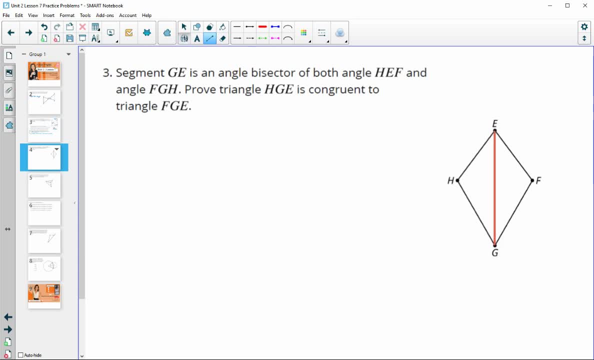 So this segment here bisects. both angles Prove that triangle HGE is congruent to FGE. So we know that since GE, GE is a bisector, let's say is the angle bisector. Well, we can probably just say: is the bisector of angle HEF. that 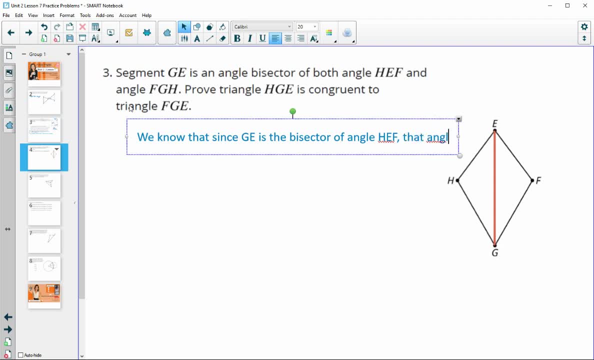 So we know, since it's the angle bisector, that angle HEG and FEG are congruent. So we know that, since it's the angle bisector, that angle HEG and FEG are congruent. GE is also the angle bisector of angle HGF. 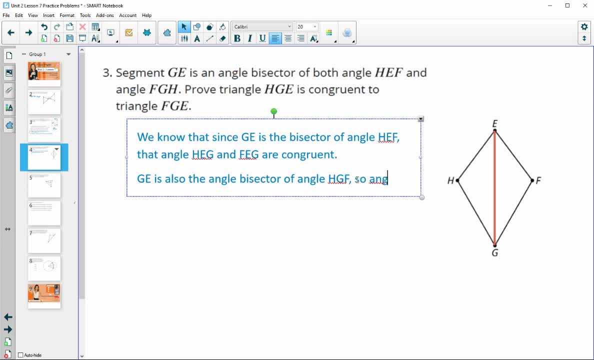 So HGE and angle FGE are congruent, And then let me mark that on the picture as we put it in there. So we got this angle. This angle is congruent to this angle and also this angle is congruent to this angle. 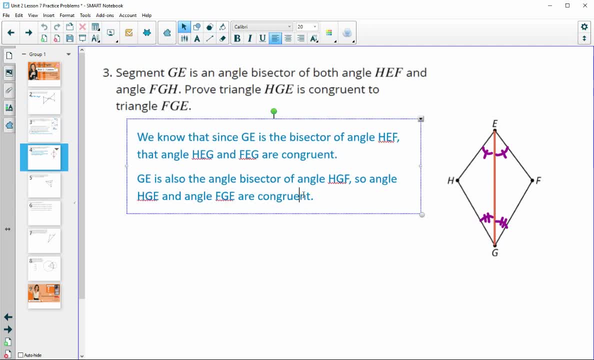 Then we also know the segment in the middle. So EG is congruent to EG because it's the same segment. We know that. Let me mark that on here, And then that's enough. And then that's enough to prove that the triangles are congruent. 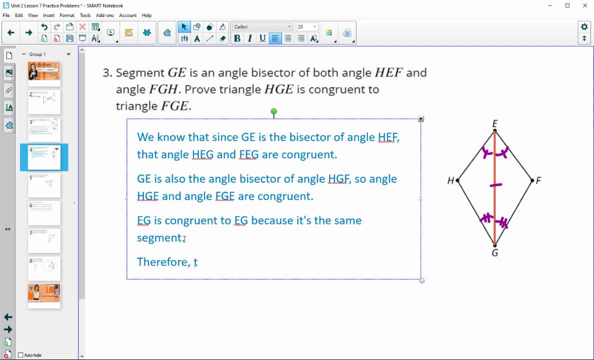 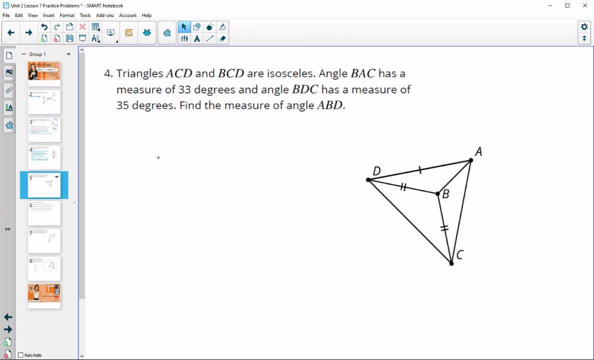 So therefore triangle HGE is congruent to triangle FGE by angle side angle triangle. congruence Number four: we have two isosceles Triangles here, So ACD, and they actually only have the one side marked here. 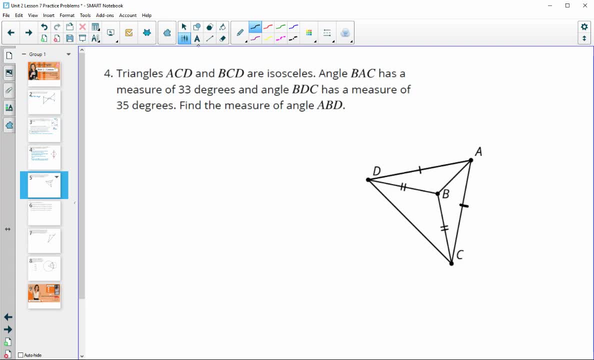 So ACD is isosceles, So this should be marked congruent as well. And then BCD, down here, is isosceles. Angle BAC is 33 degrees And then angle BDC is 35 degrees. And then it wants us to find the measure of angle ABD. 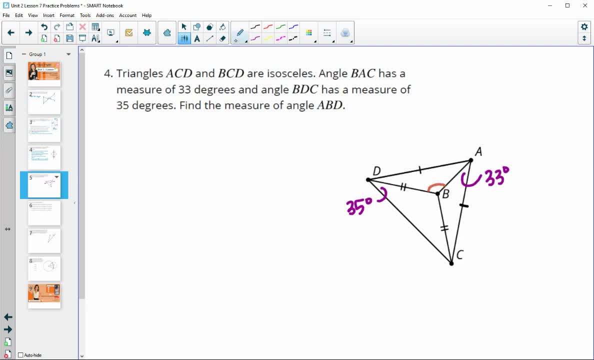 So this angle here. And then it wants us to find the measure of angle ABD. So because we have isosceles triangles, we know that the base angles are congruent. So down here this angle is congruent to this one. 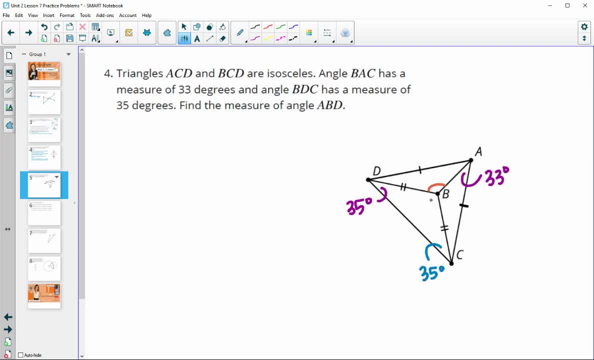 So we know this one is 35 degrees as well. So we know this one is thirty-five degrees as well, Which will actually help us find this one because we can do. the triangle sum theorem, which doesn't have 就 exactly the same name, works, because it is a breadwinner's bus period and it takes a couple hundred and ten to come up. 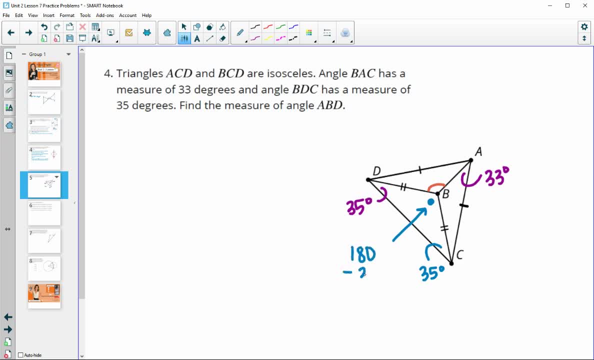 which tells us that the triangle totals 180 degrees. So we can subtract off 35 and 35 to get 110 for that angle. So this angle here is 110 degrees. And then we also know that these two triangles are the same, since they have a one tick mark and two tick mark side. 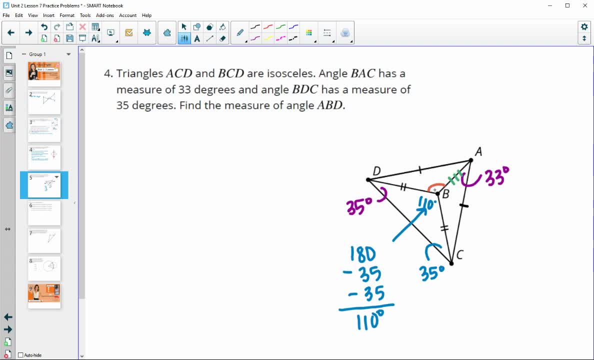 And then this side is the same in both. So these two triangles by side side side are congruent. So we know that these two angles are congruent as well And we know, right around this center, that that totals 360 degrees. So we can take 360, subtract off the 110 that we know for this angle. 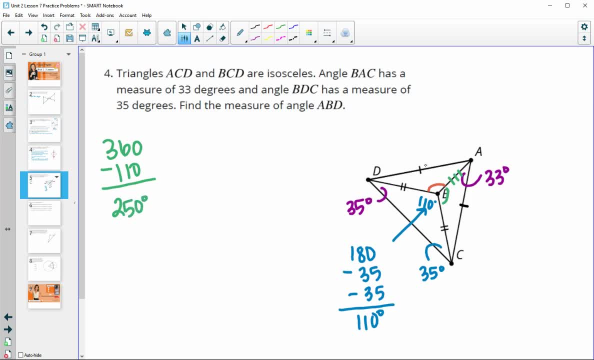 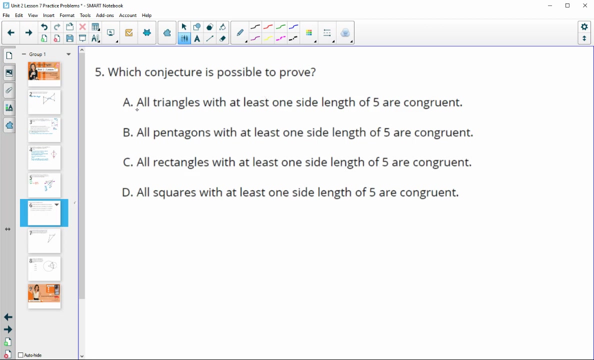 which leaves 250 degrees for these two angles, which are congruent. So then, to figure out that orange angle, we would just divide this Evenly by two, and that would give us 125 degrees for that angle. Number five, which conjecture is possible to prove? So first conjecture is all triangles. 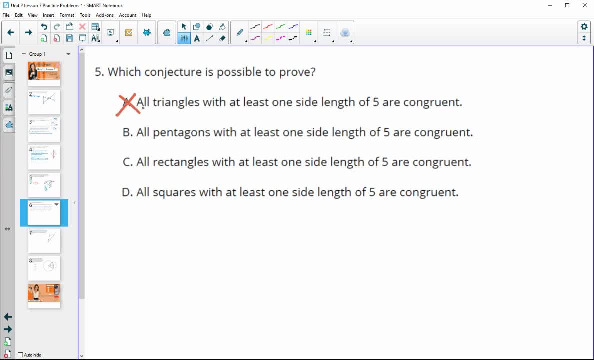 with at least one side of five are congruent. That is false. Okay, so you could certainly draw two different examples where I could put: this one is five and then I could put an equilateral triangle that all of them are five and those are definitely congruent. 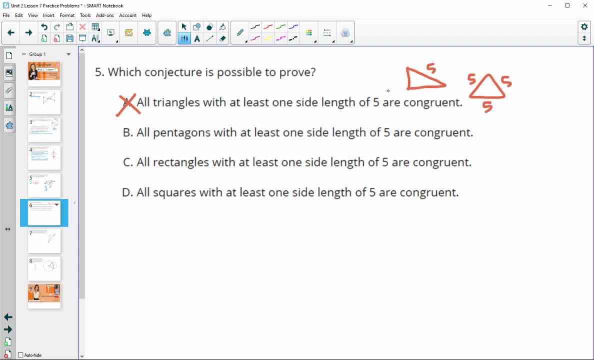 Because their angles aren't the same And these side lengths are different. All pentagons with at least one side length of five are congruent. So again, false, a very similar thing. you could have a regular pentagon where all the sides are five, And then you could just have a random pentagon. 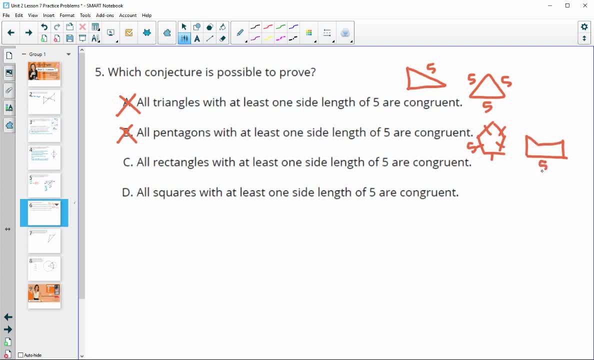 So it's that one, two, three, four, five and this side could be five, and those are definitely not congruent. All rectangles with at least one side of five are congruent. Now, with a rectangle, we do know the angles are set. So we do know that all of these angles are 90 degrees. 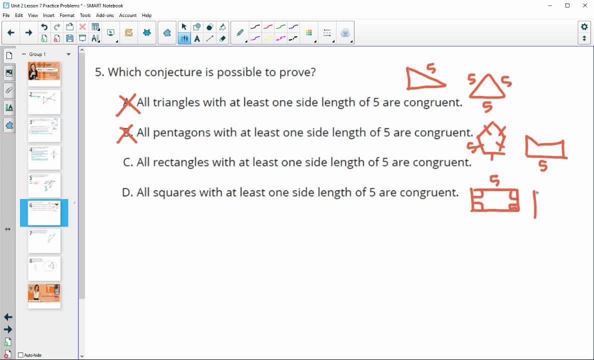 But this side could be five, Okay, and then you could also, and then these sides could be two, So you could leave it at those longer ones are five, and then this could be three, So these could each be two, these ones could be three, not going to be congruent All squares with at least 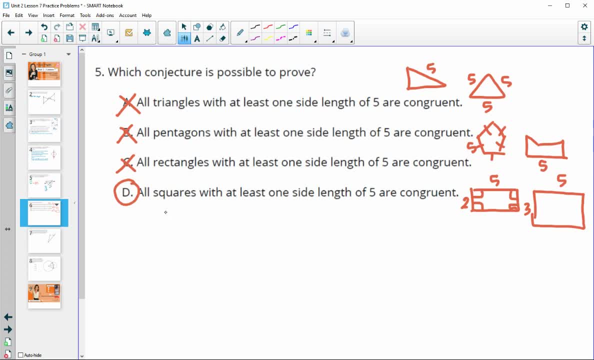 one side length of five are congruent. this would be true Because squares have their angles, are all set at 90 degrees, And then they have all congruent sides. So if one of the sides is five, all of them are five, And so if you were to read or to replicate that and draw another square, 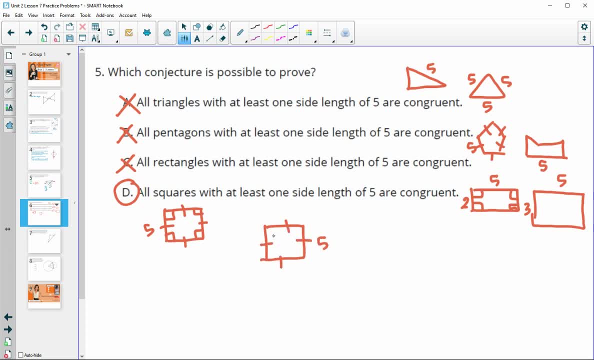 again, all the sides need to be the same. So one is five, all of them are five, and then it would also have all 90 degree angles, So all of those corresponding parts would be the same, meaning they're congruent. Number six: Andre is drawing a triangle that is congruent to this one. he begins: 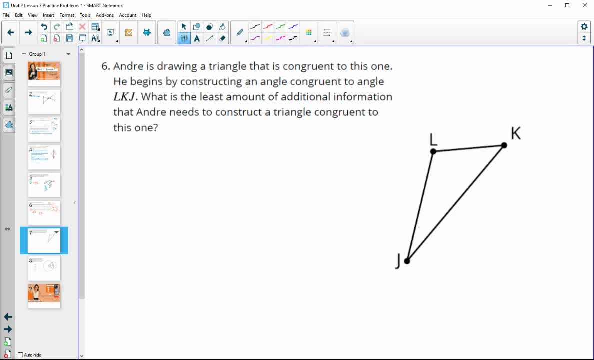 by constructing an angle congruent to LKJ. So he's created this angle so far. What is the least amount of additional information that he needs to construct a triangle congruent to this? So he needs one side length And then one more angle measure And I would say one side length, either LK or JK, So that it's 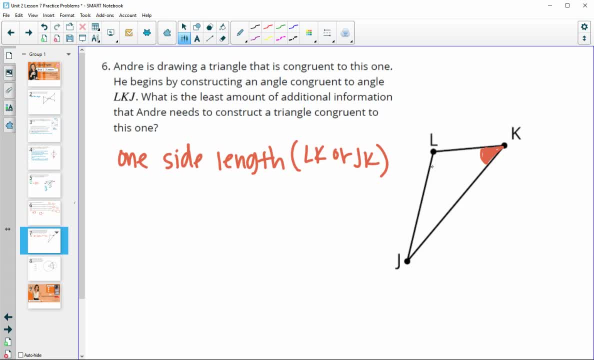 touching that angle, Not super necessary because he could get one of the other angles, but I would do one that it's touching And then one more angle measure And I would say one side length. but I personally, if I were gonna put lengths to this, so I would pick one of the side lengths that 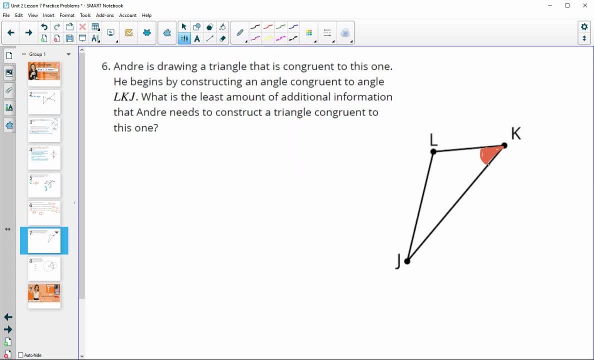 it's touching. So I would say like, just pick one LK. So I would say the length of LK And then I would pick the angle on the other side of that. So then you'd have angle side angle, so LK and the measure of angle L. 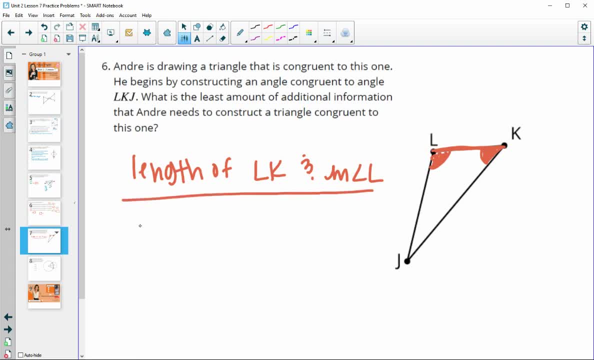 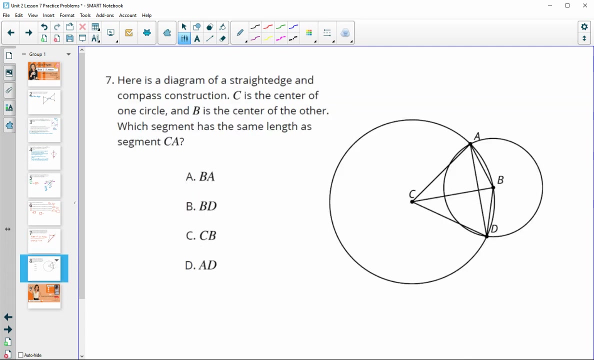 You also could do side angle side if you wanted. So you could get the length of LK and JK, So making K the included angle. So if you did LK and JK, then you'd have a side angle. side Number seven. this is a straight edge and compass construction. C is the center of this circle.